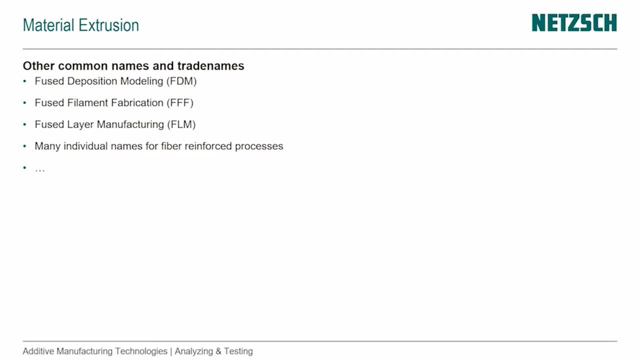 inventors of that process, often abbreviated FDM, Fused filament fabrication, FFF- that's really the open source term that's used today. Fused layer manufacturing- FLM is a terminology that's very often used in Europe, And then there are many individual names for processes. 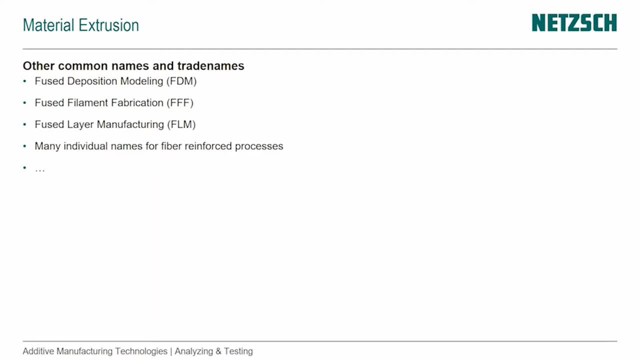 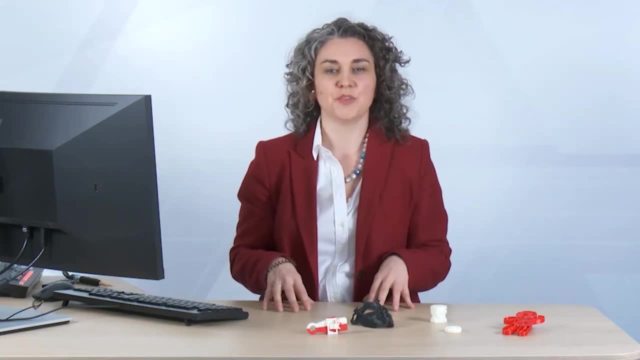 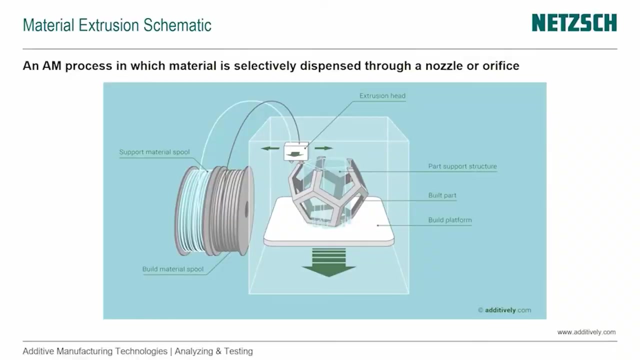 and especially for the fiber reinforced process that we'll talk at the very end. So if we look at material extrusion, we have thermoplastic materials, material that's dispensed through an orifice and we create these parts. So if we look at 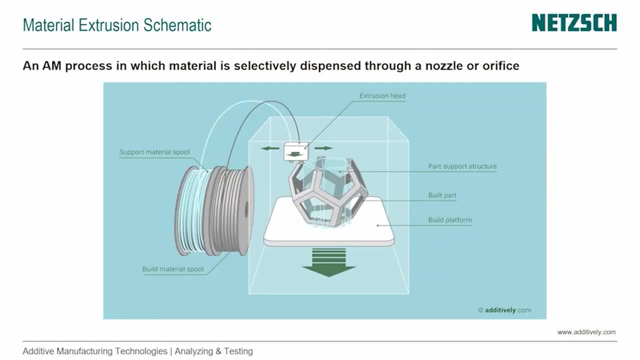 the schematic, you will see we have a build platform that's moving down. We see already depicted the build part and we see that we need support structure for overhangs in this part. And then key is the extrusion head. So that's a heated head where you can feed. 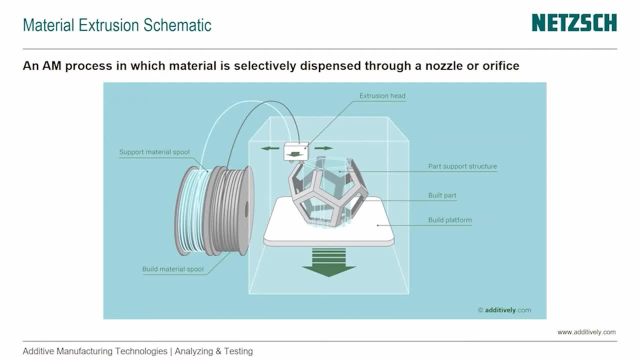 up to two materials in. There can be two different building materials, Or one support material and one build material, And this is fed through two different nozzles in the extrusion head And the extrusion head, depending on what material it's currently. 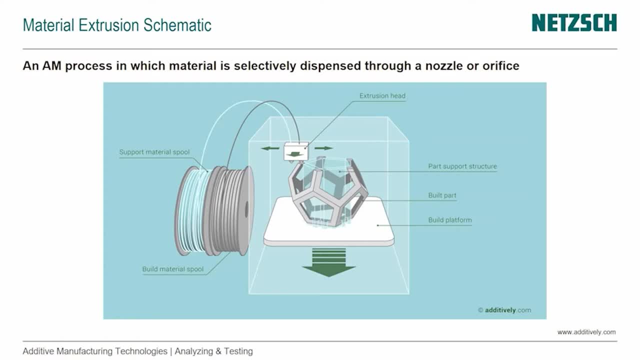 supposed to be depositing, pushes the nozzle of the material down a little bit and starts extruding the cross section of the layer. Once it has finished the whole layer, it either moves to the second material- if we're using two, Repeats that process and then it lowers down, Or, if we only have one material, we're just. 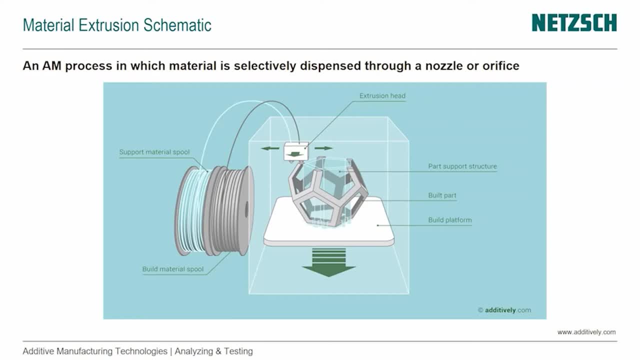 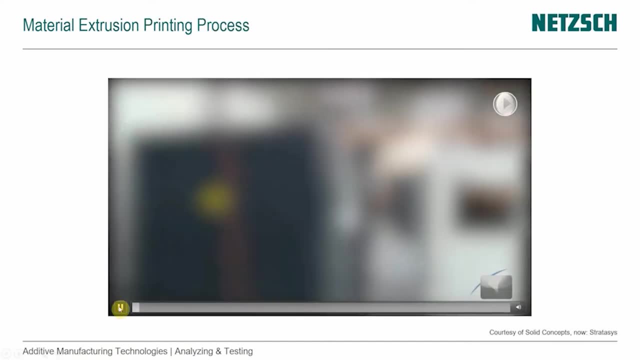 using that one material, creating the cross section, lowering down and starting on the next layer. I also have a video for you that shows the process in more detail. It's also from Solid Concepts. You've seen a couple of their videos before And this: 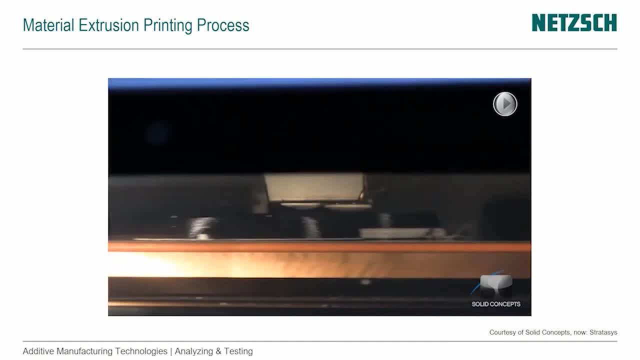 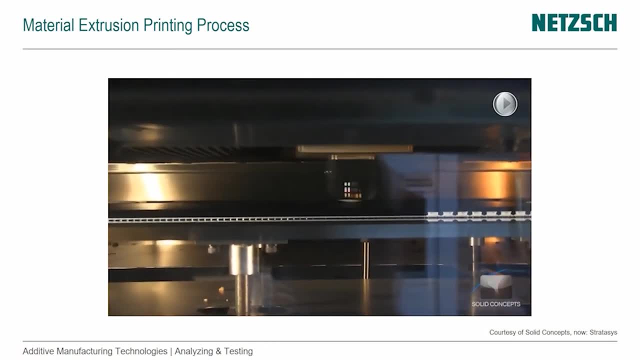 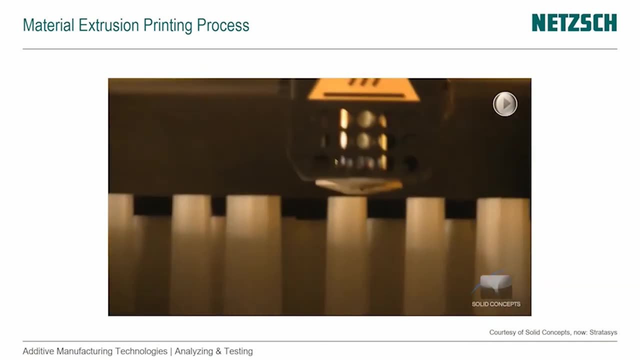 is really a manufacturing facility And you see the black being printed is the built material and the white is the solid And the black is the soluble support. Here you see it printing And you see it's going relatively fast, but also selectively deposits materials, So it has to fill a cross section.